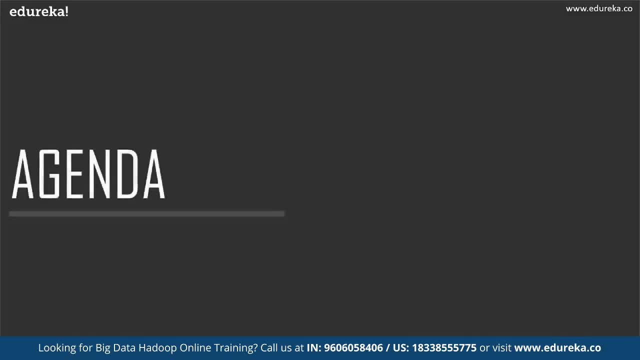 So, before moving further, let us have a quick look at the agenda for today's session. first, We will know what exactly is big data and what exactly is AWS. Then we will figure out why big data in AWS. moving on, We will discuss how AWS can solve the big data challenges. 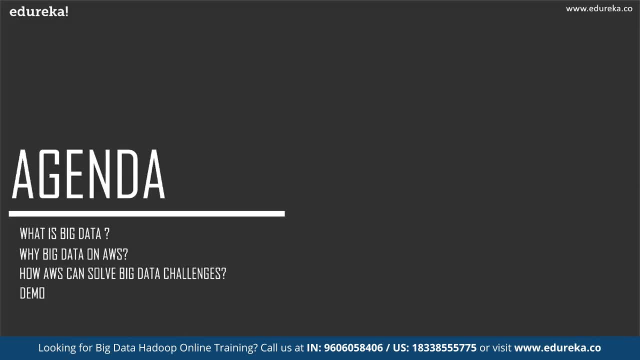 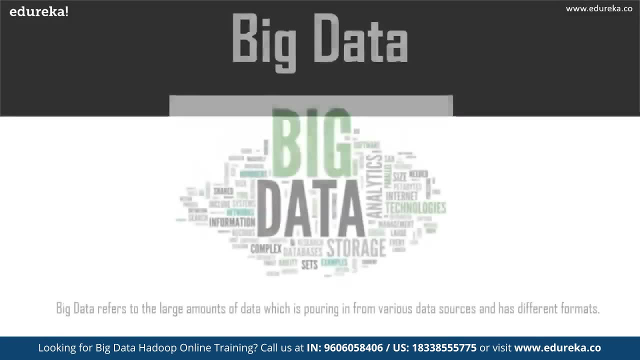 And then, finally, we will conclude with a demo. I hope I'm clear with the agenda guys. Okay, so let us begin with our first topic. What is big data? You can consider big data as high volume, high velocity and or high variety information assets. 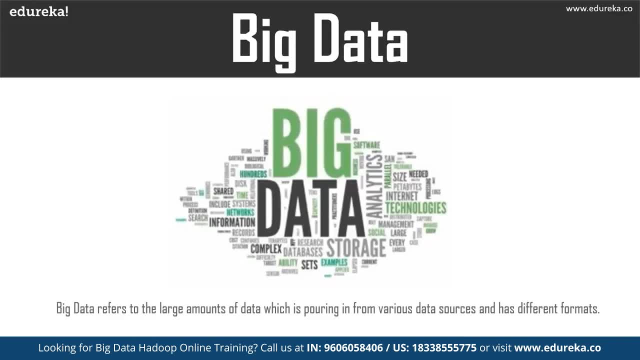 that demand cost-effective, innovative forms of information processing, and this enables enhanced insight, decision-making and process automation. So big data comprises of five important V's, which define the characteristics of big data. So let us discuss these one by one before moving to AWS. So, as you can see on the screen, 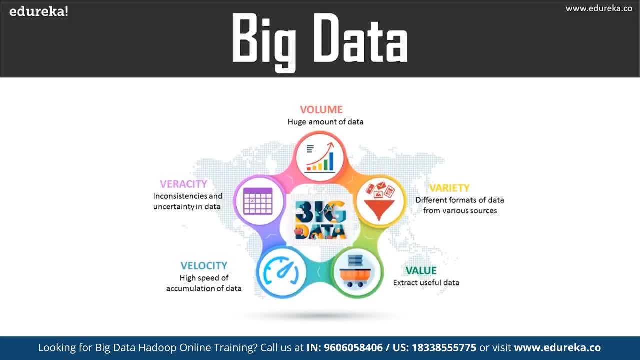 these are the five V's of big data's. the first one is the volume, which corresponds to the amount of data that is generated every day. So many of us must be aware that social media generates a lot of data. e-commerce websites also generate huge amount of data. 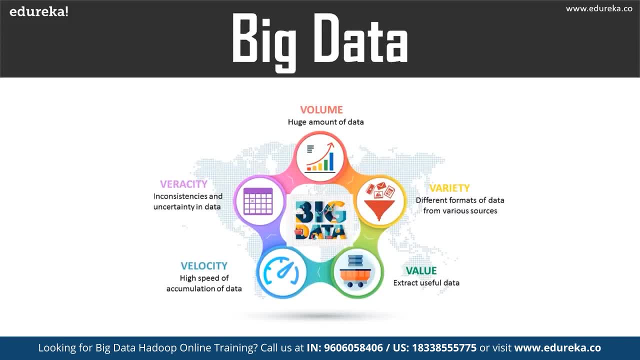 So these are the some sources that generate huge amount of data, and next is the variety of data. So it's not that data comes only in one format, So data can be structured, unstructured or semi-structured. and the next V is the value. 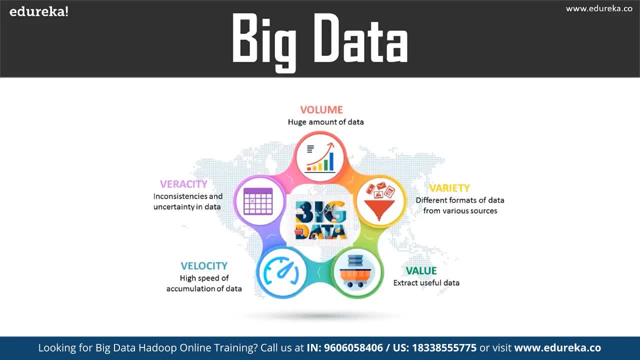 If you are not able to derive any value out of your data, then there is no use of such data. and the next V here is the velocity. So velocity here refers to the speed of data generation. and the final V in this big data is the veracity. 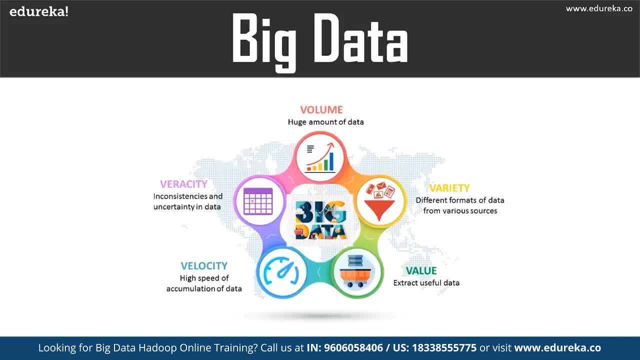 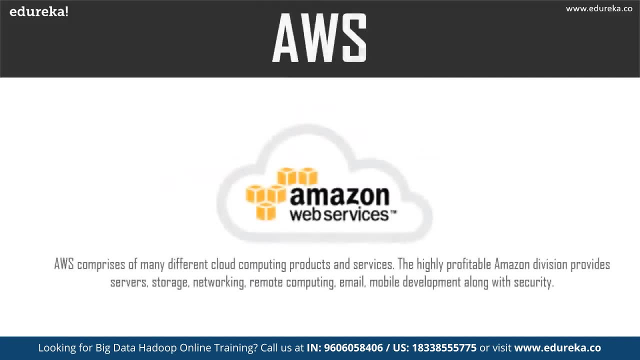 So veracity is nothing but the inconsistencies and uncertain. it is in the data. So these are the five V's that are associated with big data. Now let us talk about what exactly is AWS. AWS comprises of many different cloud computing products and services. the highly profitable Amazon Division provides servers, storage, networking. 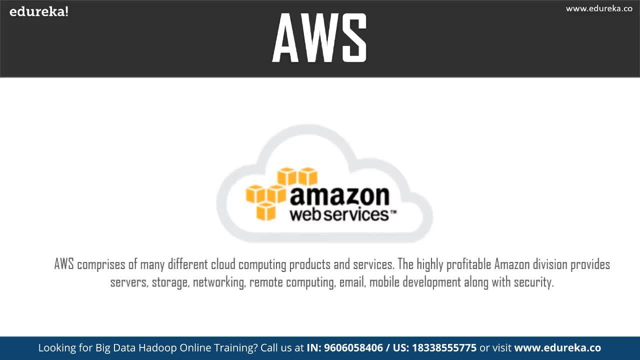 remote computing, email, mobile development, along with security. Furthermore, AWS consists of two main products: the EC2, Amazon's virtual machine service, and S3, a storage system by Amazon. It is so large and present in the computing world that it is now at least 10 times the size. 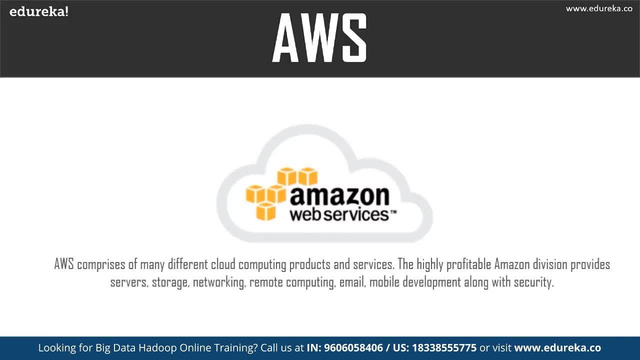 of the nearest competitor and hosts popular websites like Netflix and Instagram. AWS split into 12 global regions worldwide, Each of which has multiple availability zones in which its servers are located. these serviced regions are split in order to allow users to set geographical limits on their services. 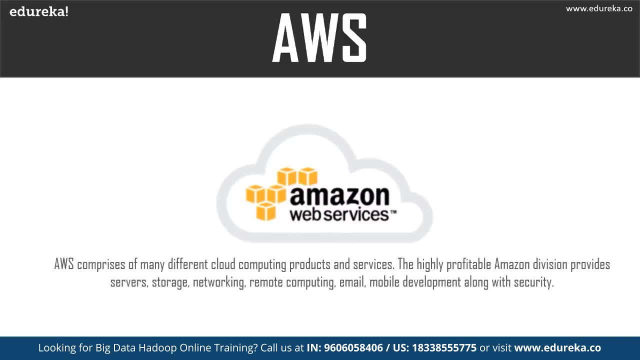 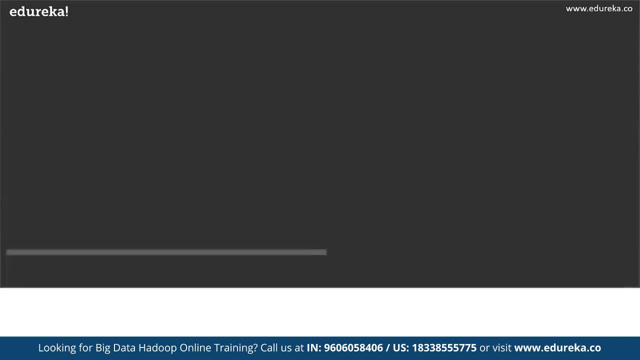 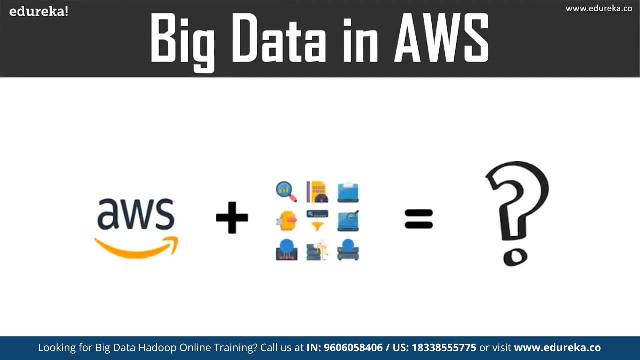 but also to provide security by diversifying the physical locations in which the data is held. So this was an overview of what exactly is AWS, and now let us talk about why big data in AWS. scientists, developers and other technology enthusiasts from many different domains are taking advantage of AWS to perform big data analytics. 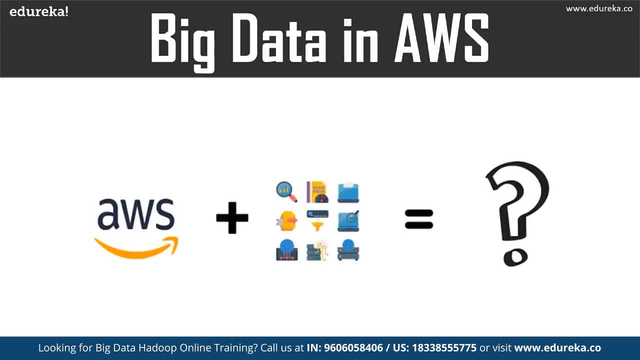 and meet critical challenges of the increasing V's of digital transformation. AWS offers you a portfolio of cloud computing services to help manage big data by significantly reducing costs, scaling to meet demand and increasing the speed of innovation. furthermore, It helps you build, Secure and deploy your big data applications. 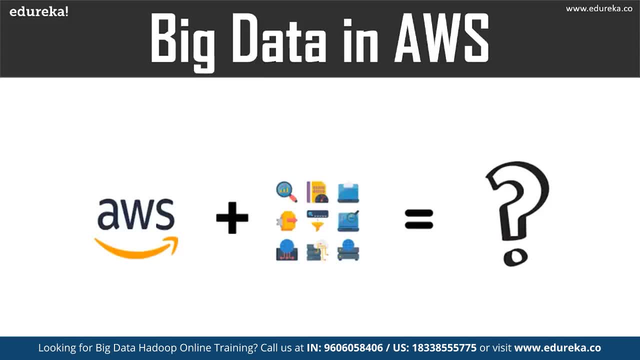 Also with AWS, you don't need hardware to procure an infrastructure to maintain and scale. due to this, You can focus your resources on uncovering new insights. since new features are added constantly, You'll always be able to leverage the latest technologies without requiring to make long-time investment commitments. 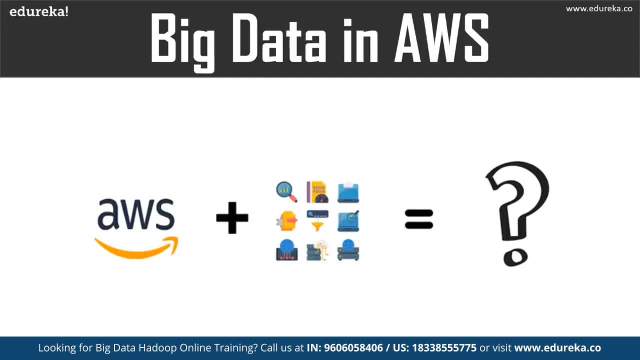 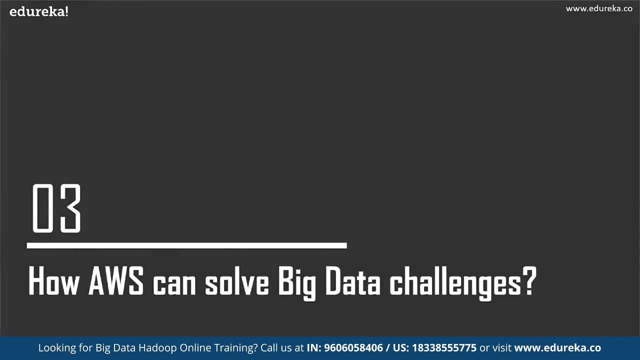 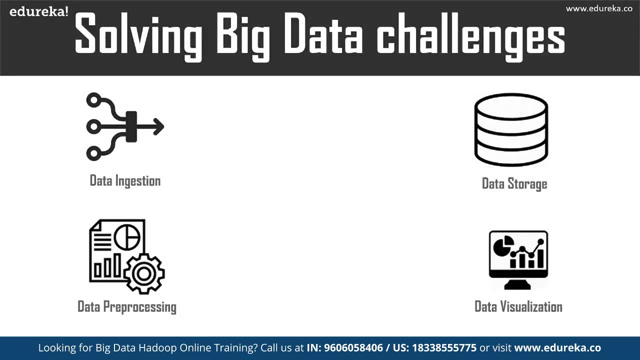 So these were the reasons why AWS and big data are perfect companions. Now let us talk about how AWS can solve the big data challenges. So AWS has numerous solutions for all the development and deployment purposes. also in the field of data science and big data, AWS has come. 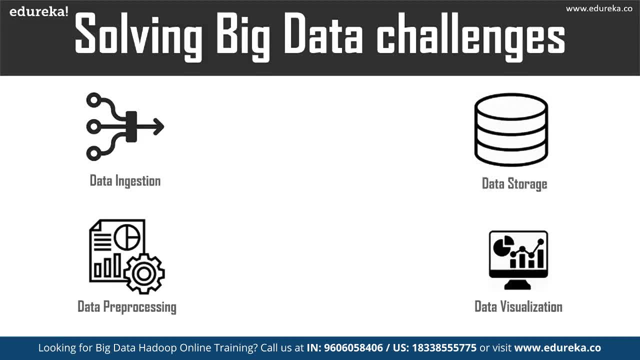 up with recent developments and different aspects of big data handling. before jumping to tools, Let us understand different aspects of big data for which AWS can provide solutions. So, as you can see on the screen, these are the various services That are provided by AWS for big data analytics. 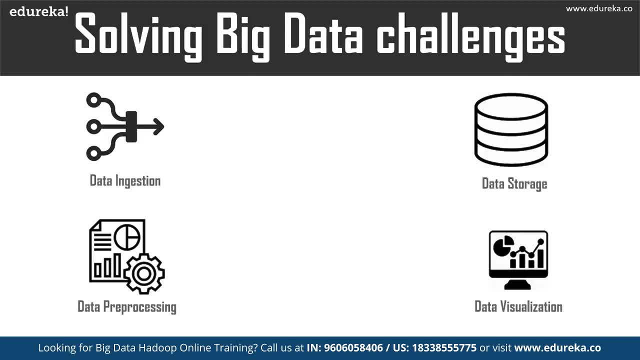 The first one is the data ingestion. So data ingestion is nothing but collecting the raw data, which can be transactions, logs, mobile devices and more, and this is the first challenge many organizations face when dealing with big data. a good big data platform makes this step easier, allowing developers 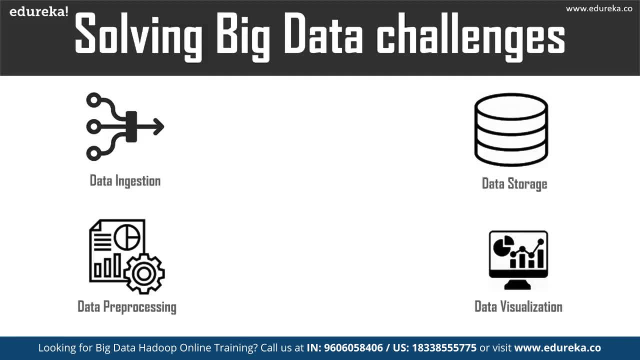 to ingest a wide variety of data, from structure to unstructured, at any speed, from real time to batch. and the second service provided by AWS is the data storage. any big data platform needs a secure, scalable and durable repository to store data prior to, even after processing the tasks, depending 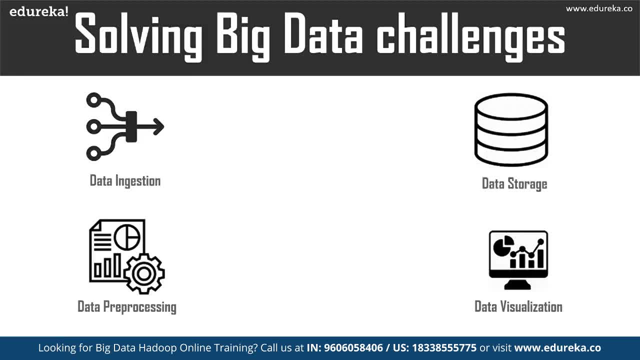 on your specific requirements. You may also need temporary stores for data in transit. and the third service here is the data pre-processing. This is the step by data transformation happens from its raw state into a consumable format, And this is usually done by means of sorting, aggregating. 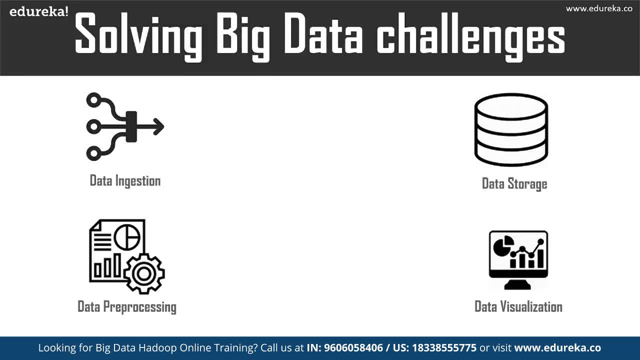 joining and even performing more advanced functions and algorithms. the resulting data sets undergo storage for further processing or made available for consumption via business intelligence and data visualization tools. and the fourth service is the data visualization. big data is all about getting high value, actionable insights from your data assets- ideally, data. 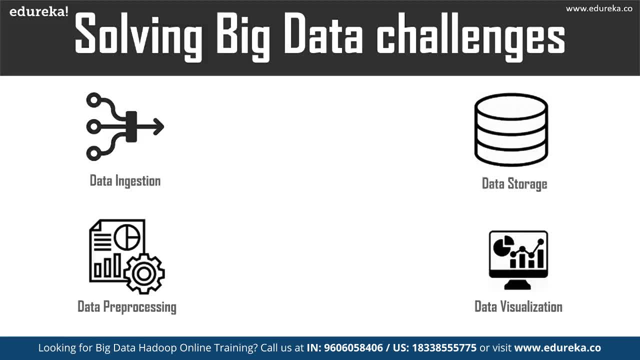 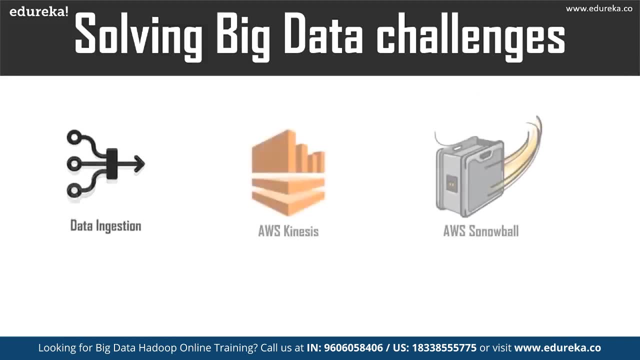 Data is available to stakeholders through self-service business intelligence and agile data visualization tools that allow for fast and easy exploration of data sets. So these were the services that are provided by AWS to handle big data. So now let us take a look at the various solutions provided by AWS. 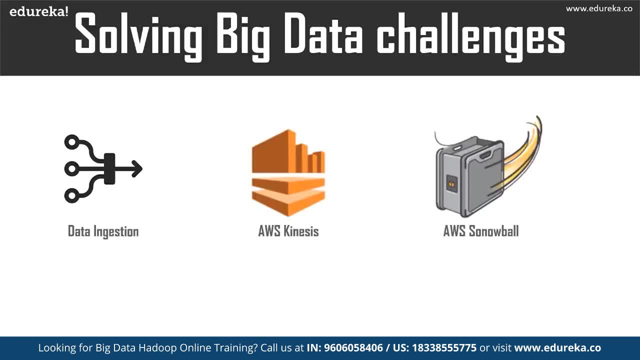 for handling different stages involved in handling big data. So the first step is the data ingestion. So for that, AWS provides two tools, namely AWS Kinesis and AWS Snowball. So if you talk about AWS Kinesis, it is a fully managed service for delivering real-time streaming data directly. 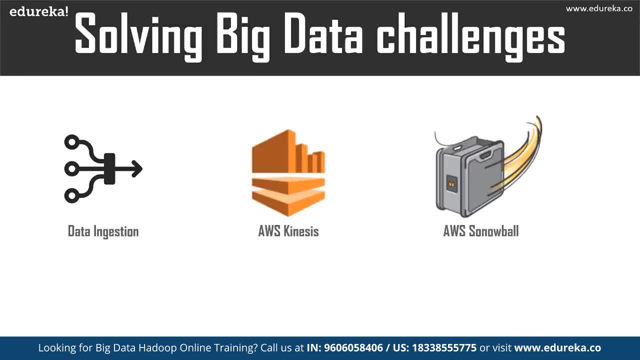 to Amazon S3. Kinesis firehose automatically scales to match the volume and throughput of streaming data and requires no ongoing administration. You can configure Kinesis firehose to transform streaming data before you store it in Amazon S3. So for those who don't know, 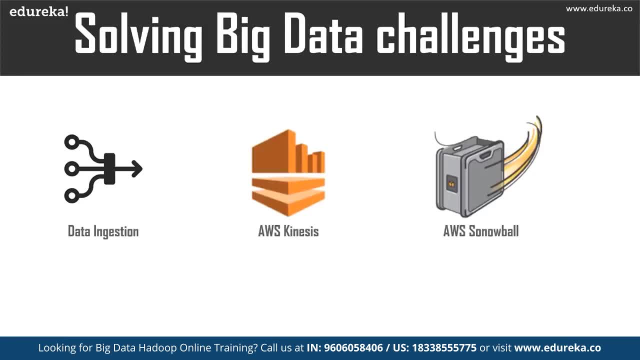 what Amazon S3 is, will be covering Amazon S3 in the later part of this session, and the next tool for data ingestion is the AWS Snowball. You can use AWS Snowball to securely and efficiently migrate bulk data from on-premises storage platforms. 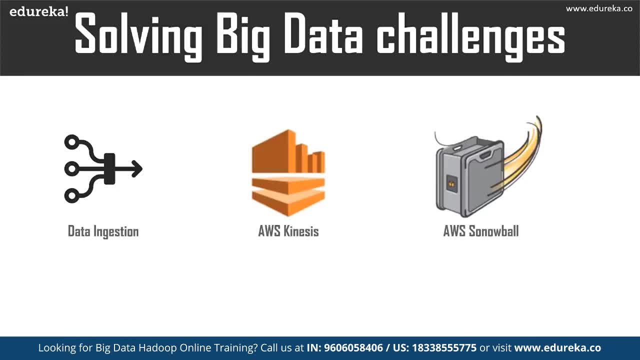 and Hadoop clusters to S3 buckets. after you create a job in the AWS management console, You automatically get a snowball appliance. after a snowball arrives, connect it to your local network, install the snowball client on your on-premises data source and then use the snowball client to select. 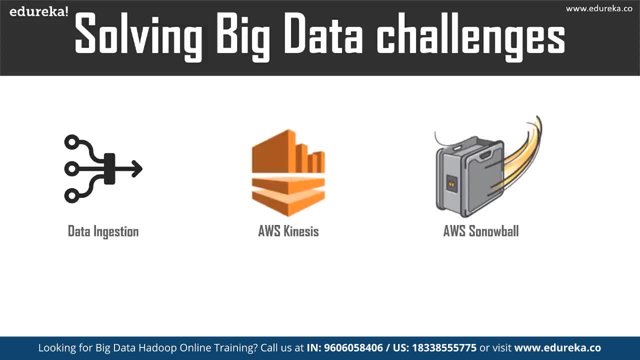 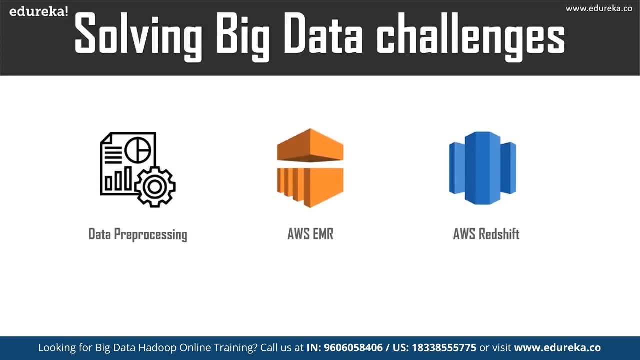 and transfer the file directories to the snowball device. So these were the tools for data ingestion purposes, And now let us talk about the data pre-processing tools. So, as you can see on the screen, the tools used for data pre-processing are the AWS EMR and AWS Redshift. 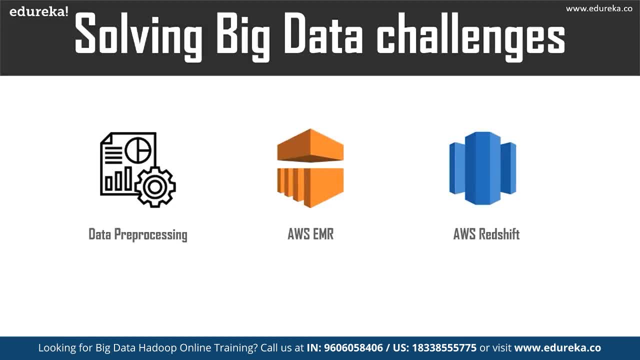 So now let us talk about the AWS EMR For big data processing using the spark and Hadoop. AWS EMR provides a managed service that makes it easy, fast and cost-effective to process vast amounts of data. Furthermore, EMR supports 19 different open-source projects. 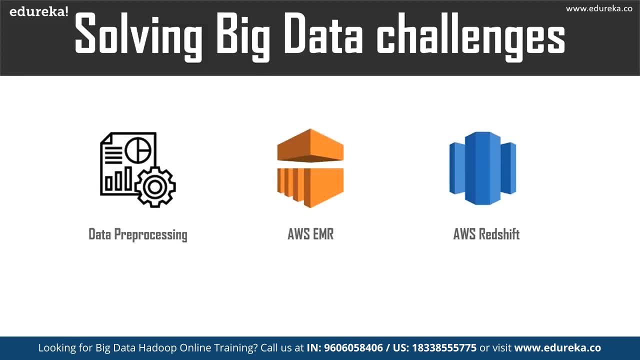 including Hadoop spark, and it also comes with managed EMR notebooks for data engineering, data science development and collaboration. and now let us talk about the AWS Redshift for data warehousing. Amazon Redshift provides the ability to run complex analytical queries against petabytes of structured data. 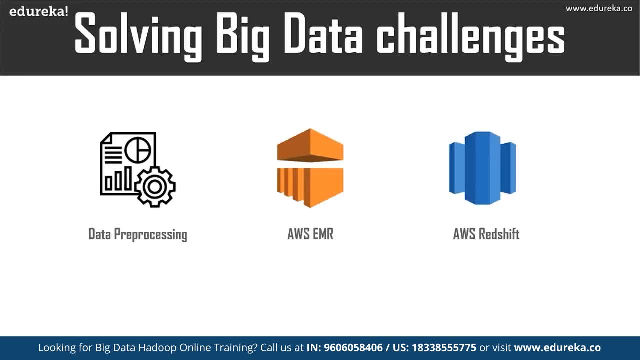 So you can just imagine the amount of data or the volume of data that can be processed by Redshift. Also, it includes Redshift spectrum that runs SQL queries directly against the exabytes of structured or unstructured data in S3 without the need for unnecessary data movement. 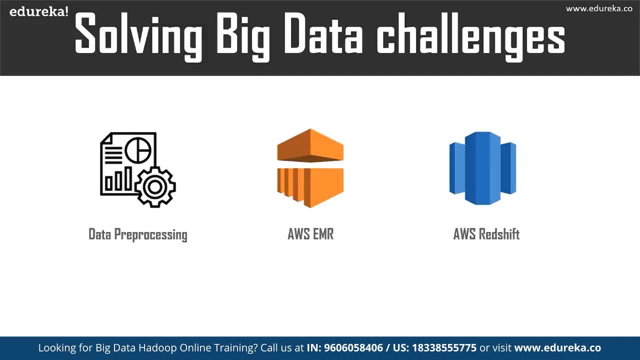 So these were the tools for data pre-processing. I hope, guys, you are understanding whatever we are discussing here. So now let us move further and talk about the data storage tools provided by Amazon Web Services. So, as you can see on the screen, there are two tools here: AWS S3 and AWS glue. 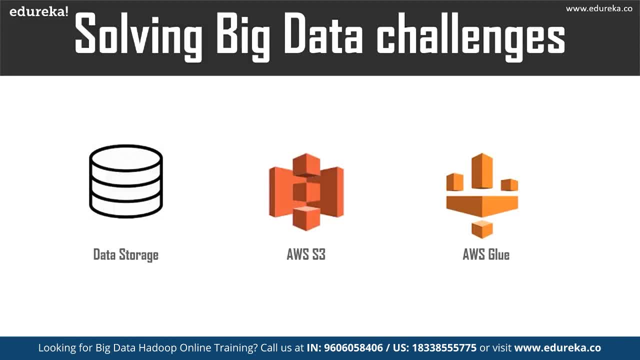 So AWS S3 is a secure, highly scalable, durable object storage with millisecond latency for data access. S3 can store any type of data from anywhere, be it website, It's mobile apps, corporate applications and data from IOT sensors or devices. It can also store and retrieve any amount of data. 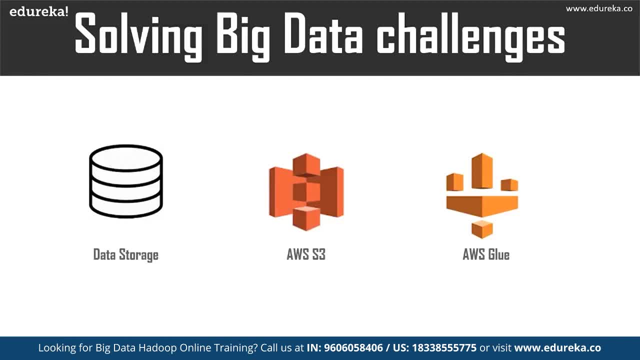 with unmatched availability and built from ground up to deliver 99.99% of durability. and the second tool here is the AWS glue. So glue is a fully managed service that provides a data catalog to make data in the data Lake discoverable. Additionally, it has the ability: 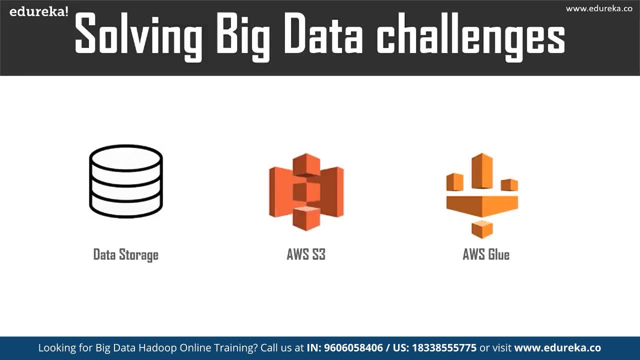 to do extract, transform and load, or the ETL to prepare data for analysis. Also, the inbuilt data catalog is like a persistent meta data store for all data assets and this makes all of the data searchable and query able in a single view. moving further, 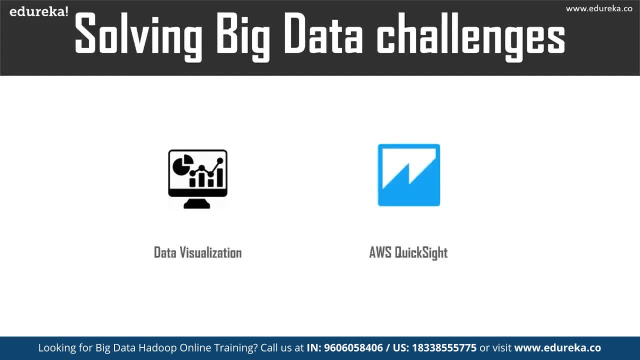 Let us talk about the data visualization tool provided by AWS. So, as you can see on the screen, for visualization purpose, the tool provided by AWS Is the AWS QuickSight. so for dashboards and visualizations, AWS QuickSight provides you fast, cloud-powered business analytics services. 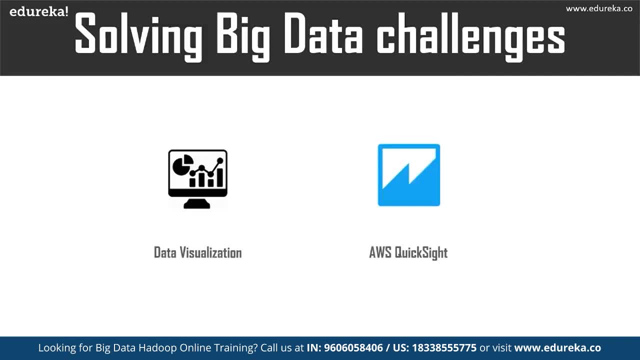 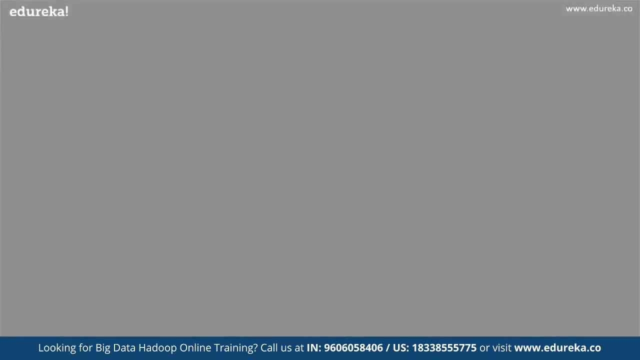 It makes it easy to build stunning visualization and rich dashboards. Additionally, you can access them from any browser or mobile devices. So these were the tools that can help you solve any big data challenge for your project, And now we have come to the final part of this session. 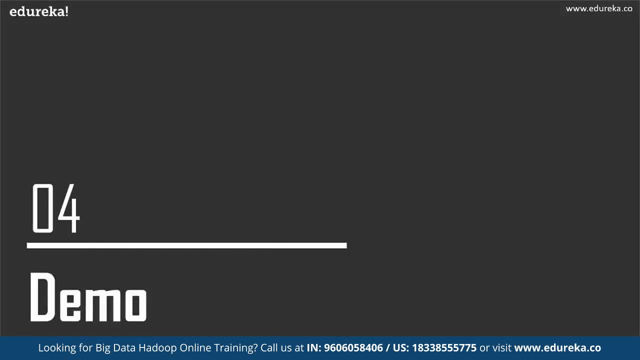 which is nothing but the demo. So in this demo we will use sample data of endangered plant and animal species from the states of Australia. here We will create an EMR cluster and configure it to run multi-step Apache Hive jobs. The EMR cluster will have Apache Hive installed in it. 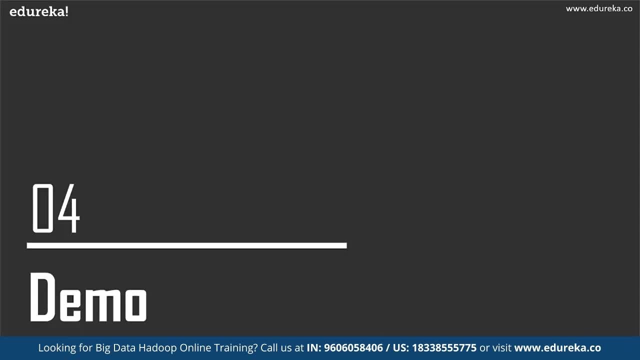 This cluster will use EMR FS or the EMR file system as the original file system, so that its data input and output locations are mapped to an S3 bucket, the cluster. We will also use the same S3 bucket for storing the log files. 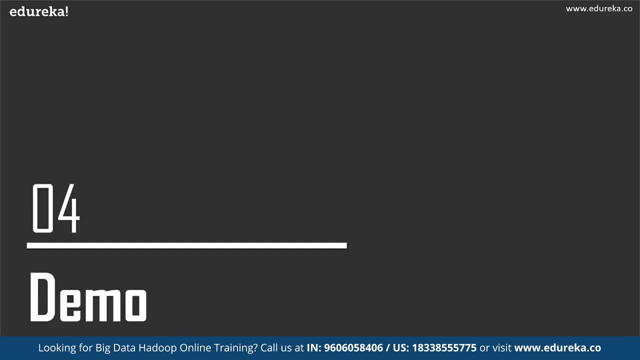 So this was an overview of the demo part that we are going to cover now. Okay, So before proceeding, guys, let me tell you you need to have a free tier account of AWS for executing this demo. Okay, So first, what we will do is I'll just quickly show you. 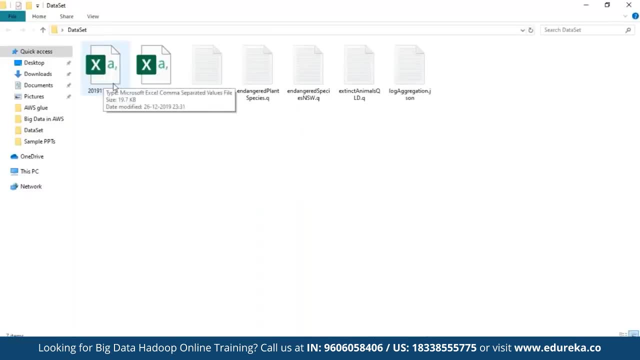 the data side that we have. So, basically, these are the two CSV files and, as discussed, we are going to run Apache Hive queries on the top of this data. Okay, So these are the queries. So for that I've created a text file. 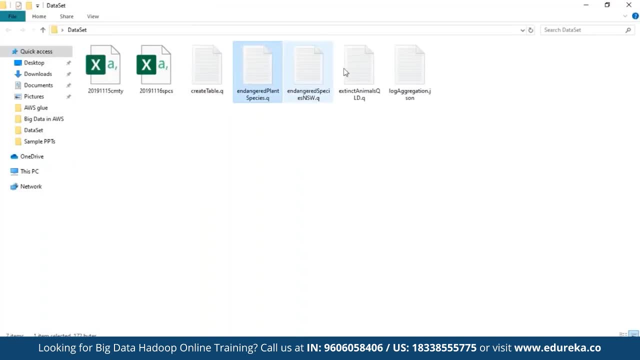 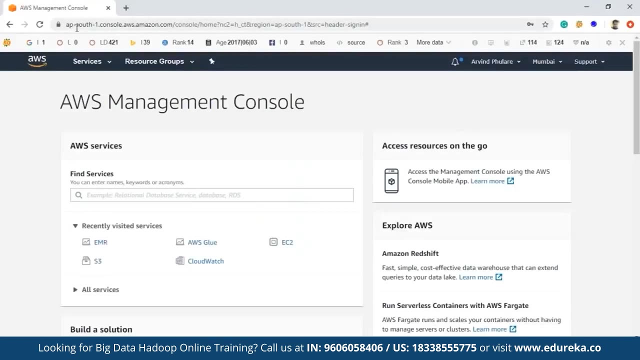 and we'll just be uploading these text files on the AWS. Okay, so let me just show you how do you do this. So for that, if you sign into the AWS management console, here in the services, you can click on storage, and here you should click on S3.. 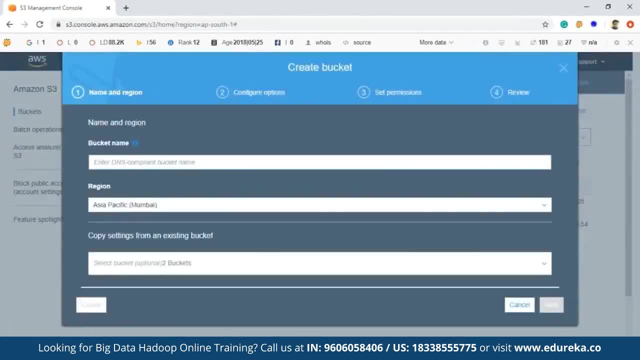 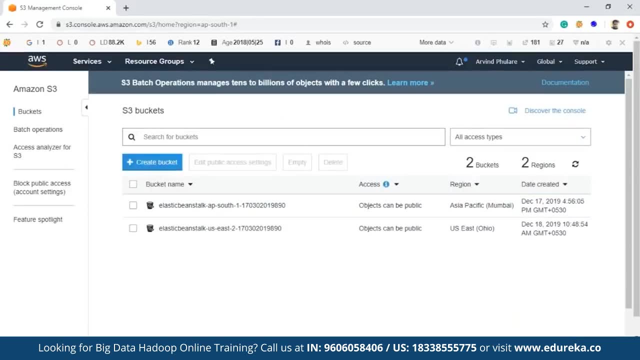 So S3 will be using for storing our data. So once you come on the S3 home page here you can see the option of creating a bucket. Okay, So now we will click on create bucket here. enter the name of the bucket, anything that you want to say, for example: 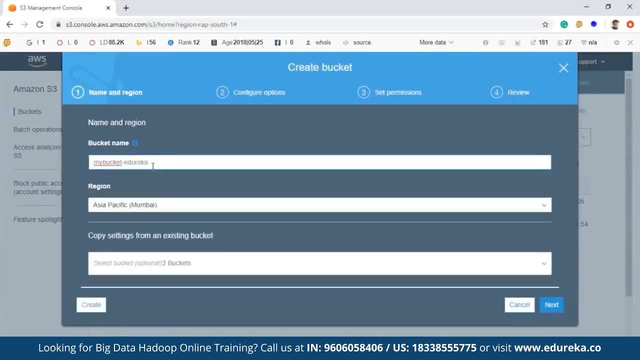 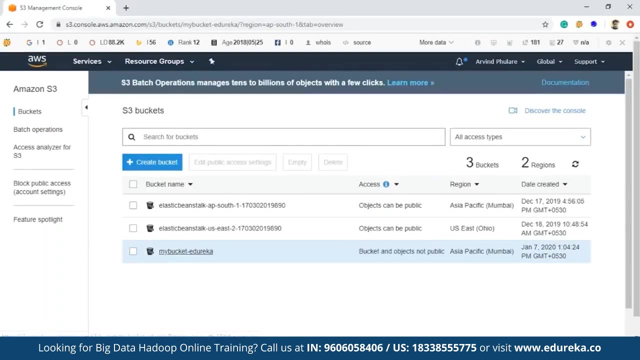 my bucket and edureka specify a region here, So I'll be selecting this one: Asia Pacific, Mumbai, and here you should click on create. So, as you can see here, this bucket has been created, my bucket, edureka, So now click on this bucket. 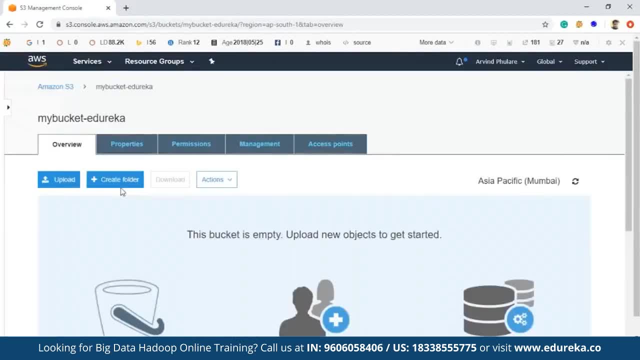 and we have to create So four folders here. Okay, so the first folder will be input, for storing the input files and after creating a cluster and running the queries. So whatever the output will be generated, It will be stored in the second folder. 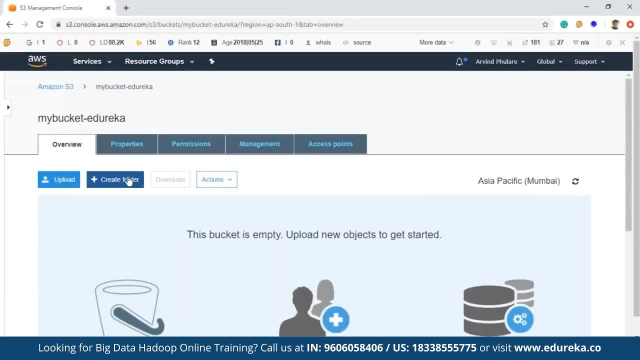 which is the output folder. The third folder is the log folder, which will consist the logs, and the purpose of log files is to debug the Apache Hive queries, like if you are running a query and if there is an error in executing that query. So for that purposes, for resolving such errors. 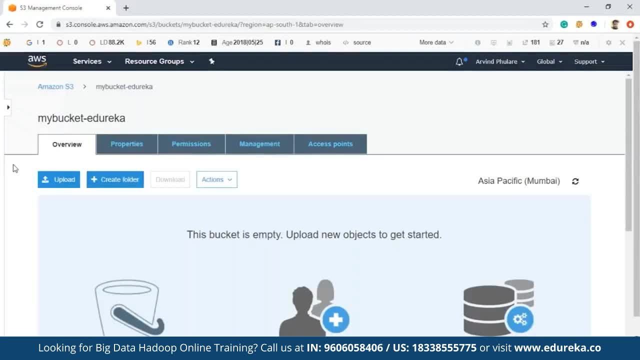 we can make use of the log files. and the fourth folder is the script where we will store all our queries in the form of dot-q files. Okay, so let's just create quickly create folders for folders. First one is input, name the folder as input and click on save. next, 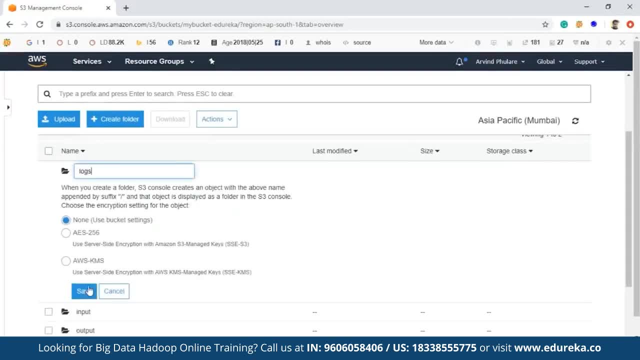 We will create the output folder on save. the third folder is the logs folder and the fourth folder is the scripts. Okay, so, as you can see, these four folders have been created here. Now let us click on input, And here we will upload our input files. 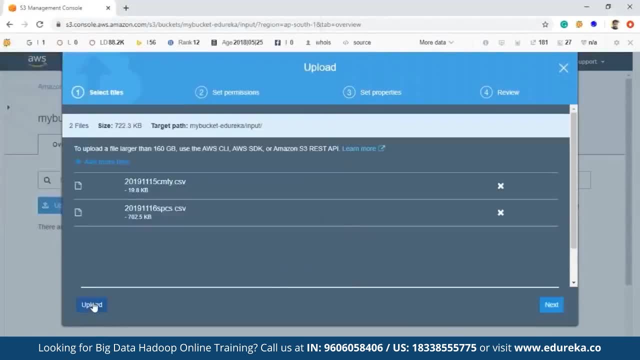 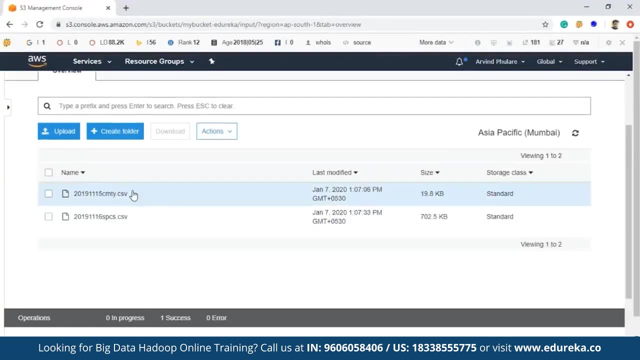 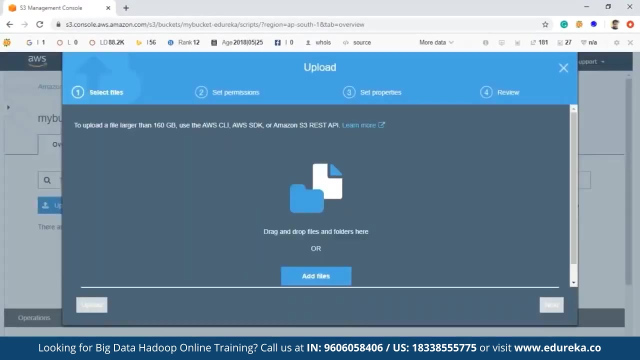 So these are the two CSV files. click on upload. So, as you can see here, both these CSV files have been added here in the input folder and now let us add scripts here. So for that, click on upload here, click on add files, and then you must browse all those. 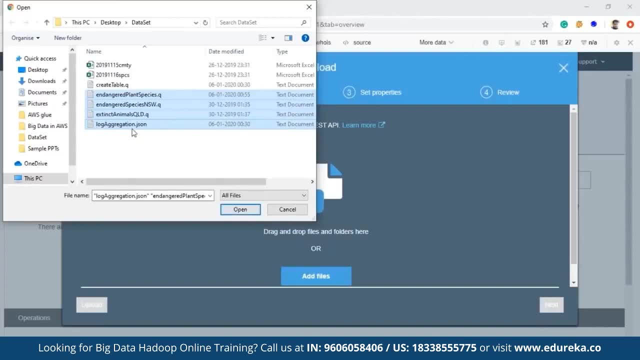 Okay. so there's also this file called log aggregation dot JSON file. We'll tell you more about this file in the later part of the video, and we must also upload this JSON file in the script folder. Okay, So, once you select all these four files, the first three files: 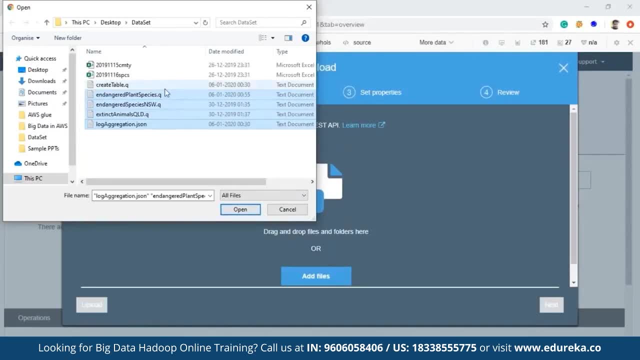 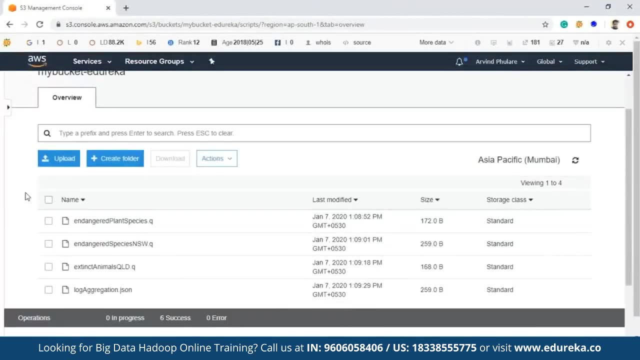 are the queries that we are going to run, and the fourth file is the JSON file. Okay, so click on open. you click on upload. Okay, says you can see here. We have added this four files here in the scripts folder of the Amazon S3 bucket. 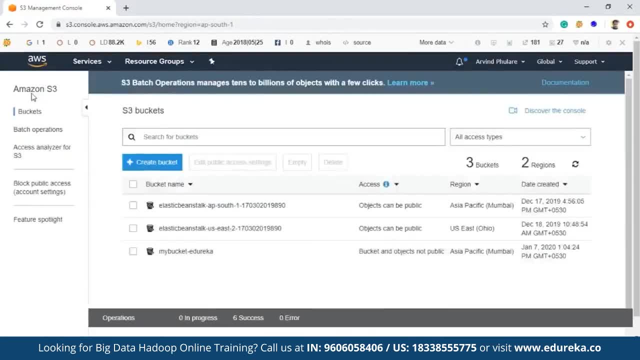 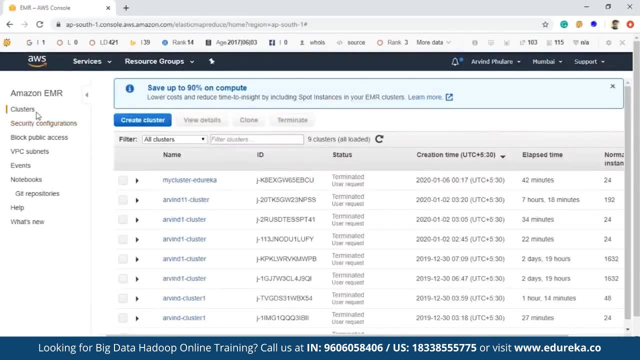 Okay, So now we are done with the S3 part of this, This demo, and now let us talk about the EMR. Okay, So here we are going to create a cluster, So for that there's an option of create cluster here. 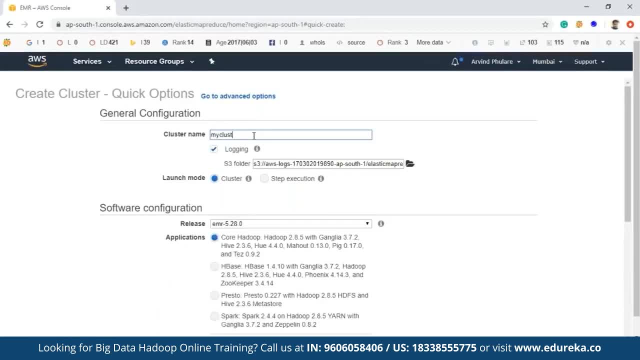 You can name your cluster whatever you want. So say, for example, my cluster at Eureka. So here you can see the option of logging. It is by default checked and, if you remember, in the previous step we created one log folder- logs folder- in the Amazon S3 bucket. 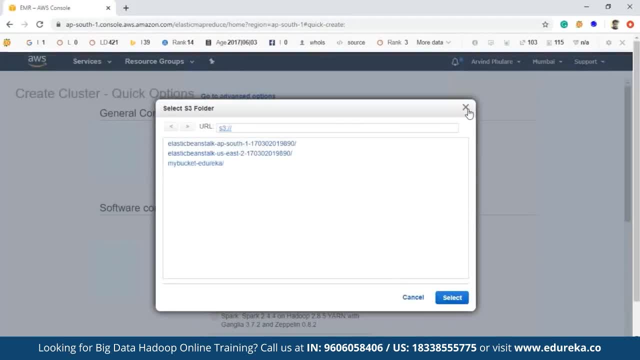 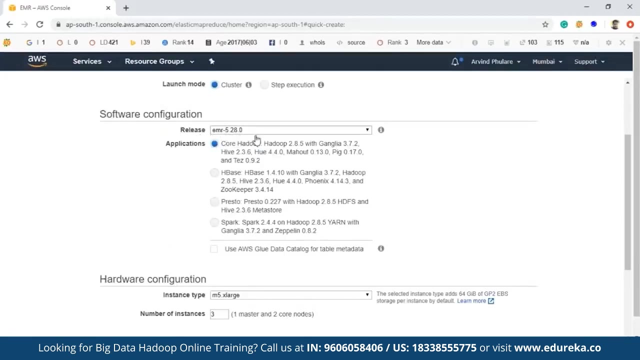 So we just need to specify that here. So for that, click on this Folder icon here and select your bucket and click on the logs folder and click on select. Okay, So this has been done here. So by default the release is EMR 5.98.0. 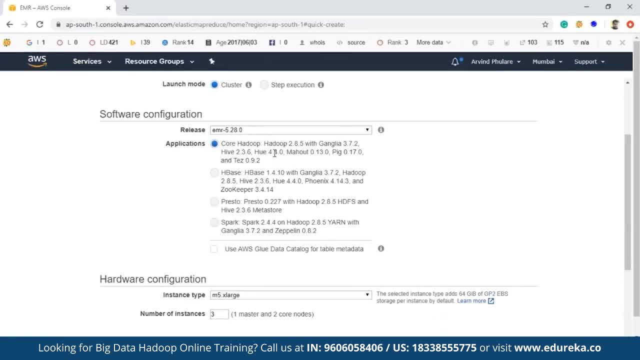 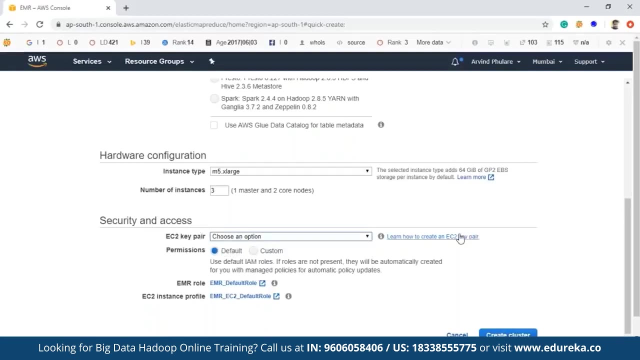 and this is the application which is selected by default. So here it has core, Hadoop, hive, who mount, and pig, along with test. So in the security and access section here there's an option of easy to keep it. So here you need to create a Amazon easy to keep it. 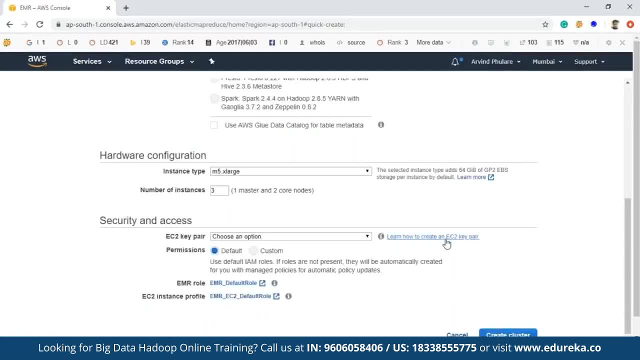 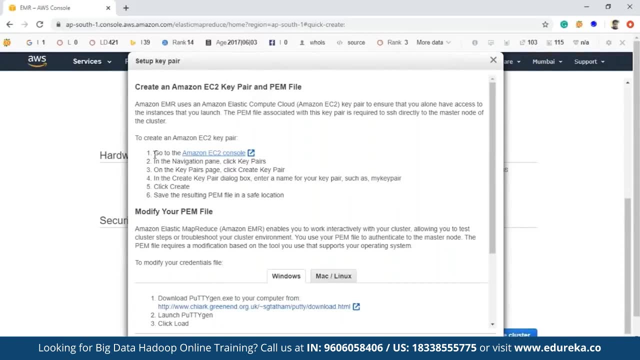 Okay. So if you click here on this link, learn how to create an easy to keep. it will show you the guidelines. Okay, So these are the steps that you need to follow to generate an Amazon easy to keep it. So go to the Amazon easy to console- click here. 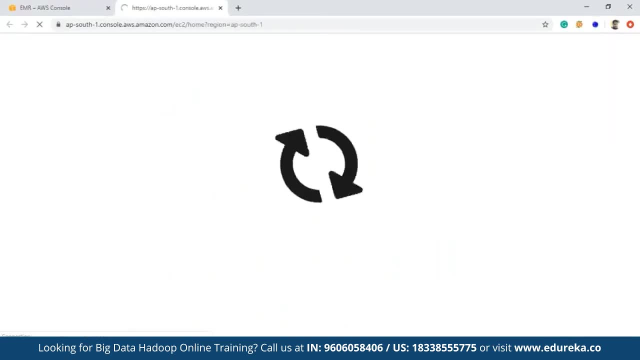 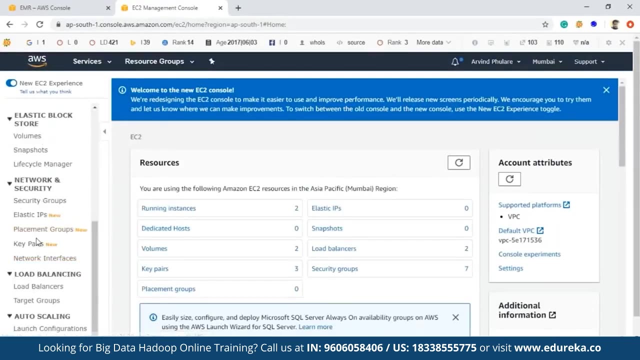 It will navigate to the easy to console. So if you see, here in the left hand side, here there is an option of key pairs: Okay, Network and security keepers, if you click on this. Okay. So these are the few of the keys. 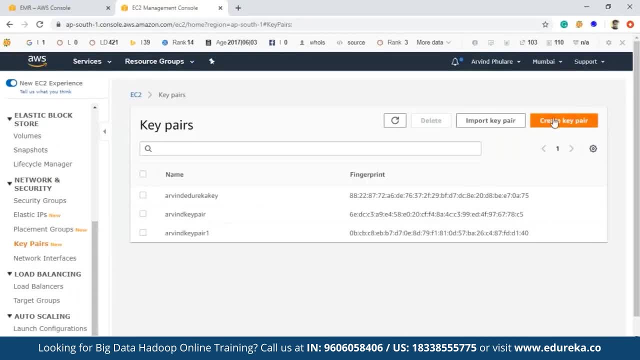 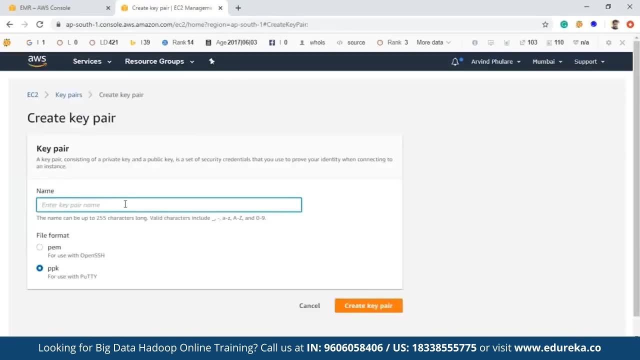 that I have already generated for my previous purposes, and now let's just create a new key pair. So for that, click on create key pair and you can name, key the key, whatever you want. my key See, for example, Edureka. so you just name it and the file format. 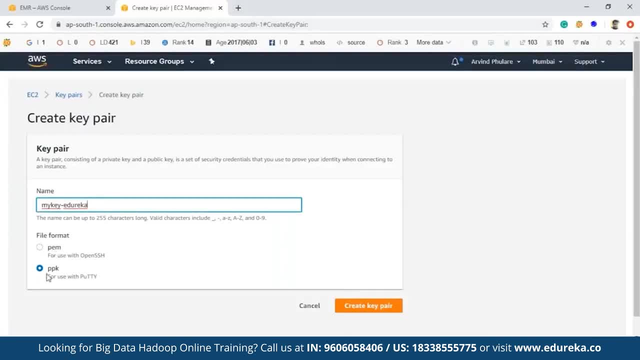 So there are two options here. One is the PEM or the PPK. So here I'm selecting the PPK for the private key. Okay, so we will talk about this PPK or the party private key in the later part of this session. 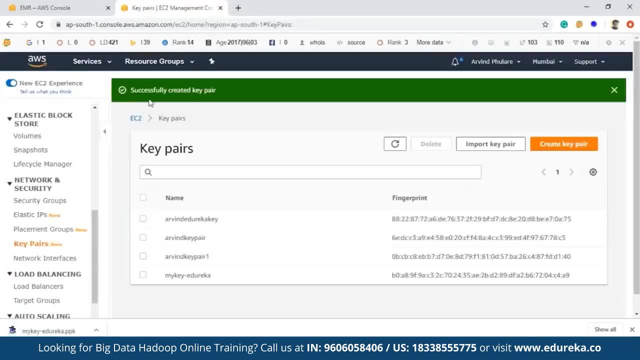 and click on create key pair. Okay, So here, as you can see, successfully created key pair and this key pair has also been downloaded on your system, as you can see here: Mikey Edureka dot PPK. So this is how you create a, easy to keep it. 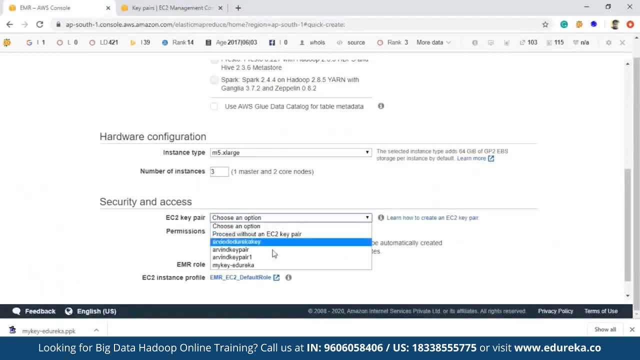 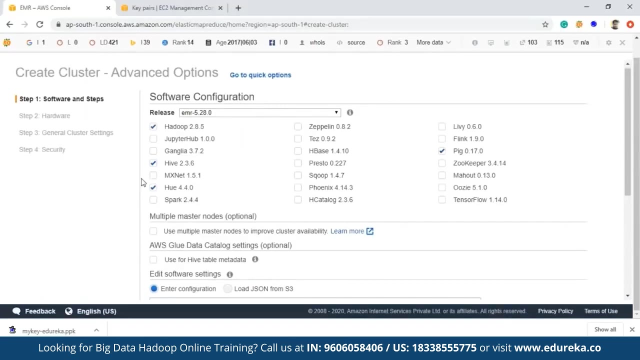 and as soon as you create this keeper, you'll have this option of choosing this: Mikey Edureka. So this was the keeper that we created just few seconds ago, So I'll just select this, Okay, and click on Advanced option here. So here, mostly, we will be going with the default options here. 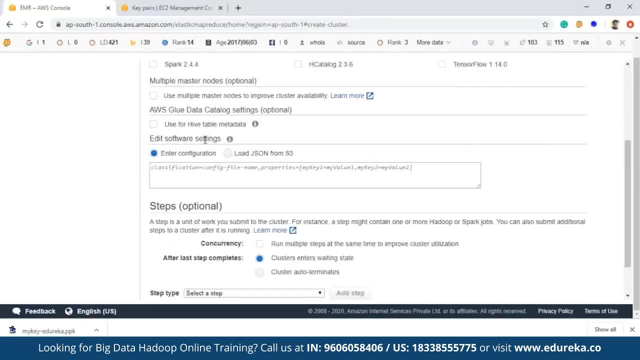 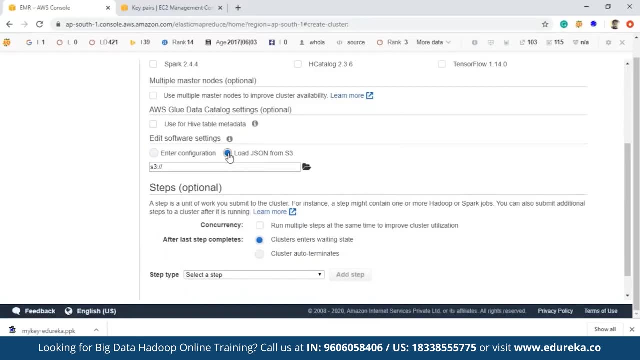 Yeah, So in this section, edit software settings, you have to click on the Jason load Jason from S3. So if you remember, we had one Jason file which we uploaded in the script folder of the S3 bucket, So we just have to navigate to that and select that file. 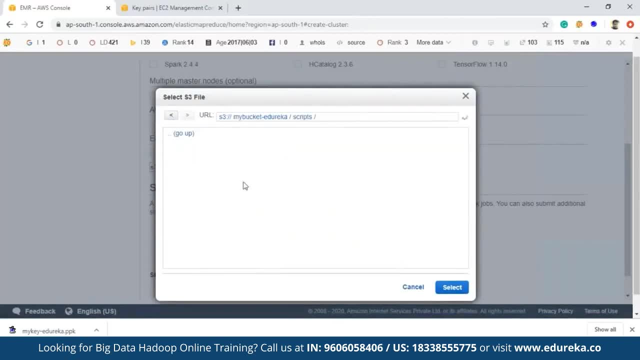 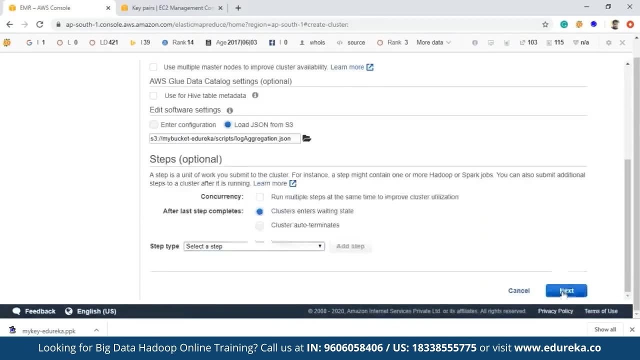 So you have to select your bucket Right here and go to the scripts folder and select this log aggregation dot Jason file. So you just have to select this here and click on next year. So here in the step 2, which is the hardware configuration, 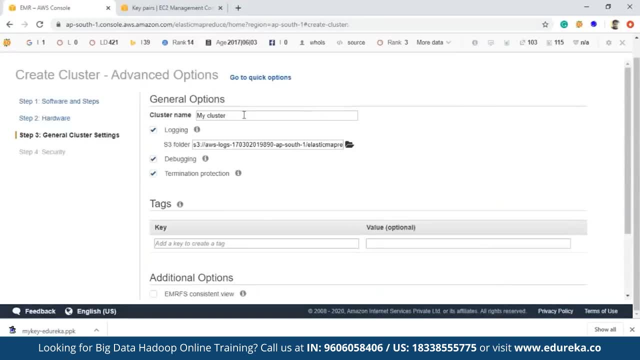 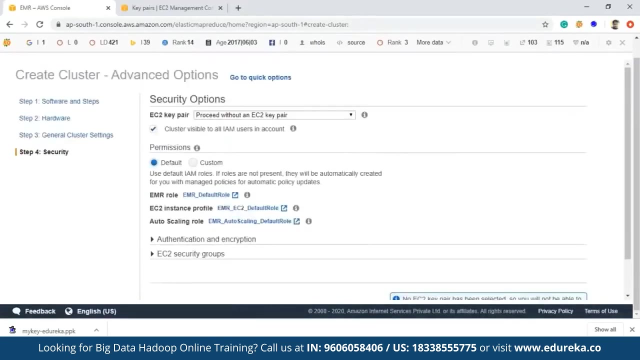 We are going with the default options. click on next. Okay, so I'll just quickly rename this: my cluster. Do you really come and select the log folder? Once you are done with this, Click on next. the fourth step is this: security here. 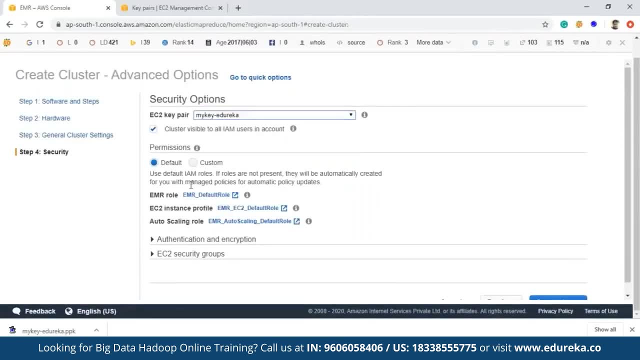 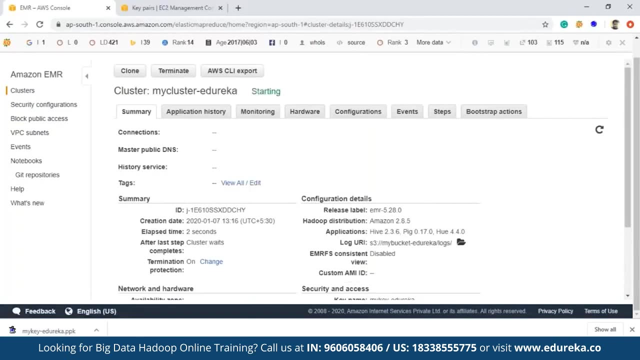 We have to select the key pair that we created and click on create cluster. Okay, so creating cluster might take a few minutes. as you can see here, it is showing the message starting. So from starting it will proceed to running and from running it will be waiting. 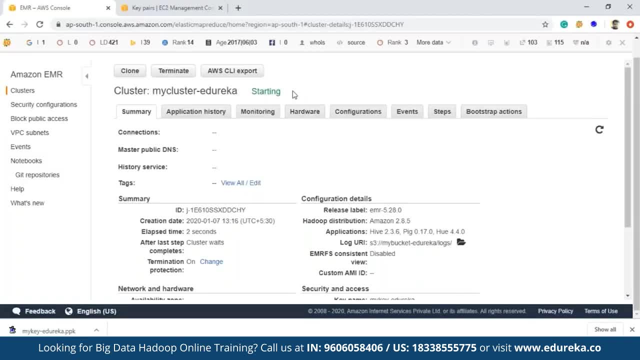 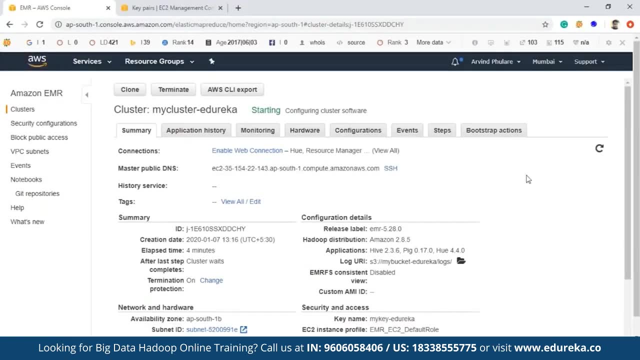 Okay, So once it enters the waiting state, then we will add steps to this cluster to process the hive queries. Okay, so the next step here is allowing the SSH access for that. What you need to do here is so. this is the cluster home page. 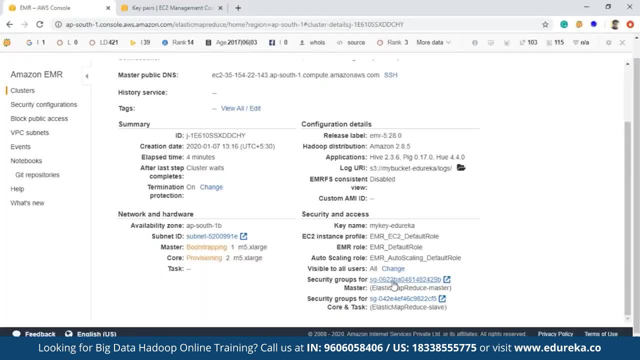 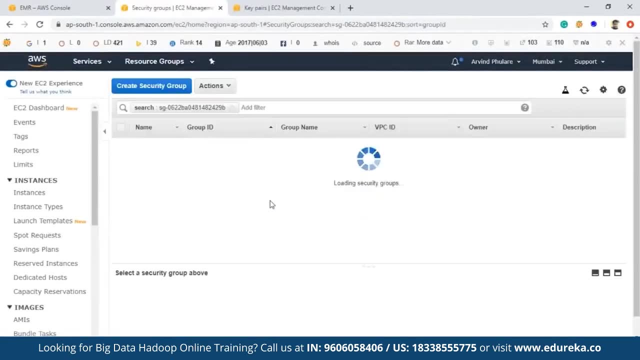 and you're in security and access. You just need to click on elastic MapReduce master. Okay, So this is the link for that. just have to click here. Okay, Once you click on that, have to select the master here: elastic MapReduce master, and here, as you can see, you have. to click on the inbound tab. after that, click on edit. So you're. what you need to do is click on add rule here and select SSH from this option type and by default it will be TCP and the port range will be 22. and here in the source, you have to click on my IP. 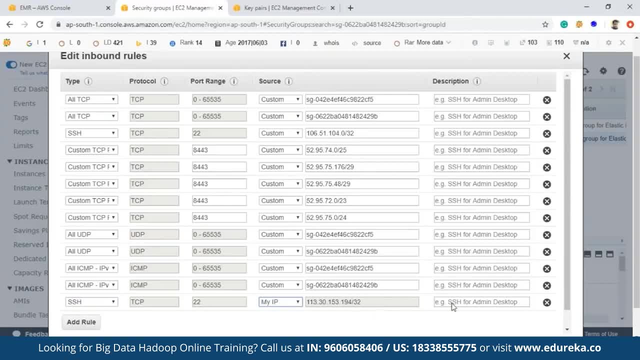 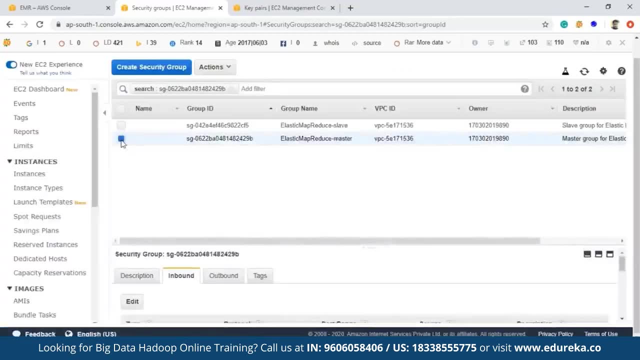 Okay, so your systems IP will appear here and you have to click on save here. So once this is done, you can do it same for the slave as well. Okay, so normally what happens in in real time cluster is nothing, but you know, there's one master. 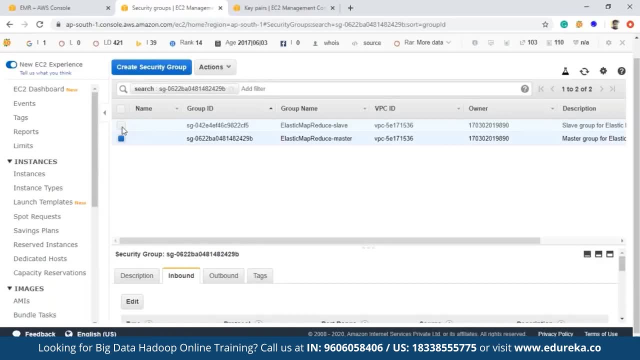 and multiple slaves. So the cluster that we have created here, It has one master and two slaves. So normally what happens is slave is a different machine and master is a different machine. But in this demo, here we the master and the slave is the same machine. 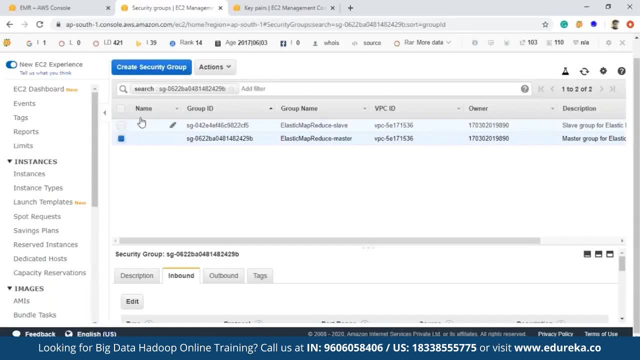 Okay, so optionally you can configure the slave as well, just as you configure the master. Okay, so it is optional and once you're done with that, you have to click here on SSH. master. public DNS is an option of SSH here, Once you click here. okay. 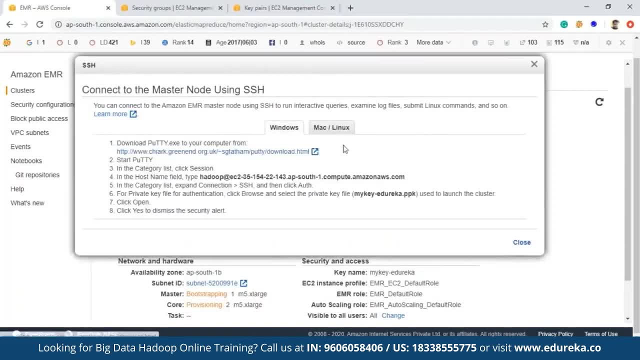 so here, depending upon the operating system that you're using, there are a few steps that you need to follow and, using this step, we can connect to the master node using SSH. Okay so, if you have Mac or Linux, you can follow these steps, and if you are using Windows OS, you can follow these steps. 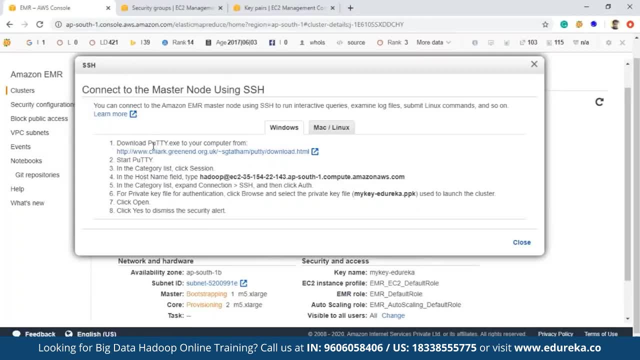 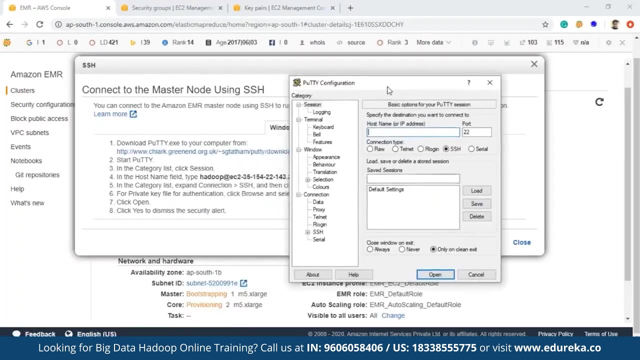 for that you'll be needing one application called party. just go on this link and download this application. So I've already downloaded this on my system, So what I'll do is I'll just quickly open that application, buty. So here it is, asking for the host name. 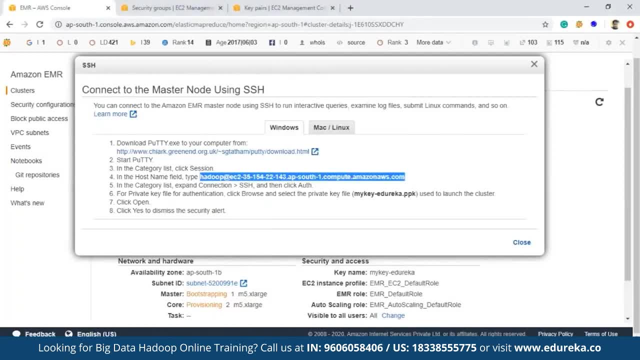 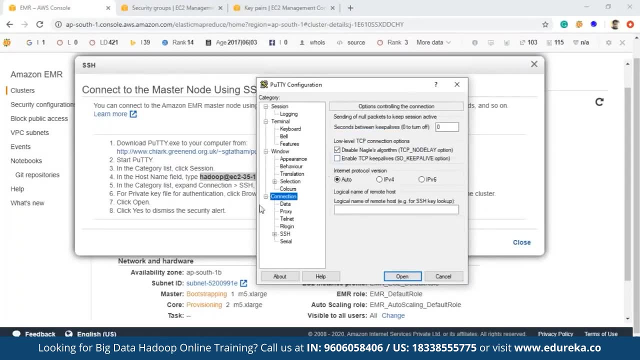 or the IP address. for that You have to select this: control C, control V. So once you're done with this, click on the connection here. after clicking on connection, you can check this box, enable TCP keep alive and then click on SSH here You have to click on the authentication tab here. 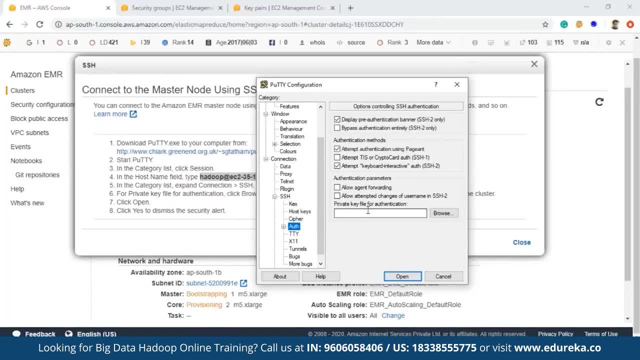 And, if you remember, we are generated one PPK file or the ec2 key pair. you just have to browse here that key from the downloads. Mikey Edureka was the name and you have to select your okay near. you have to click on open Okay. 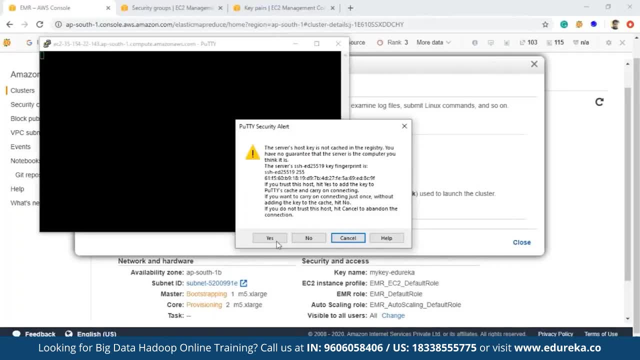 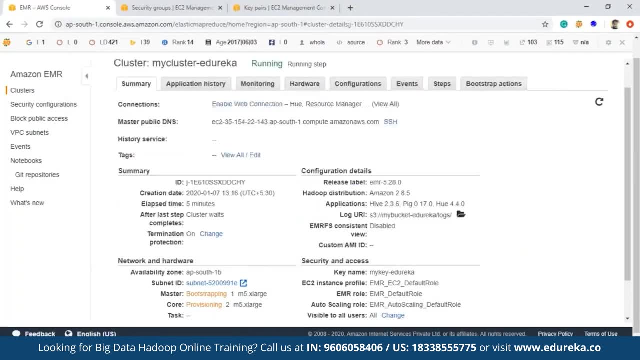 So once you do that, you'll get this message here: security alert. Just click on yes. Okay, So now we are connected to the master node using the SSH. Okay, So now our cluster Isn't the waiting state and we are good to proceed further. 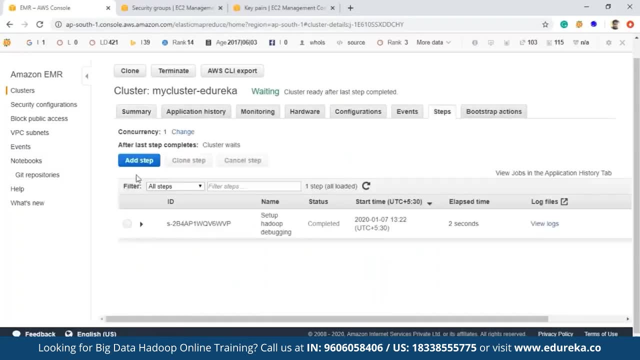 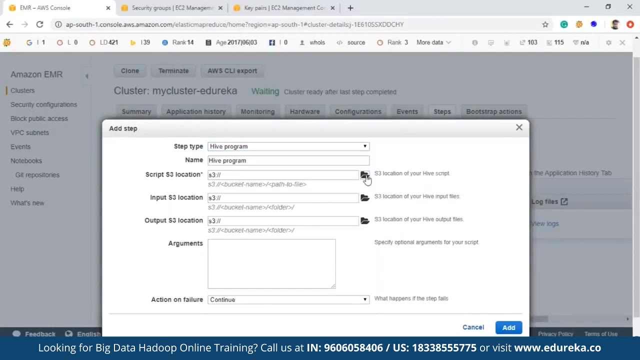 So what we will do here is here: click on steps. Okay, So basically we will be running our hive queries here. So for that click on add step in the step section, step type, select high program here and select the script for this. So for that you have to browse to the s3 bucket script. 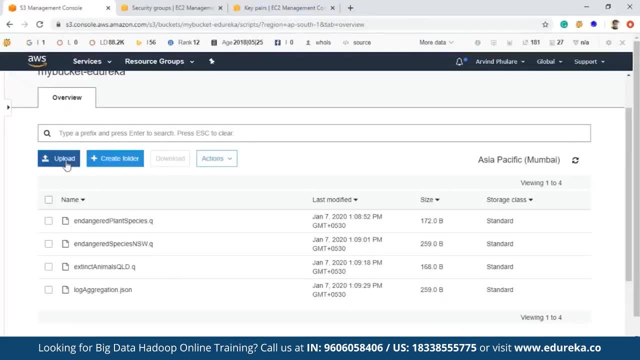 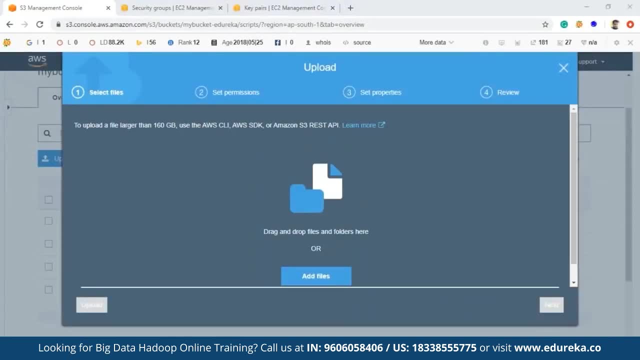 and click on. okay, guys, So I just missed uploading one more file here, So let's just quickly do that. Okay, the first query, the create table query. Let's just upload this. We are uploading this file in the scripts folder of our bucket. 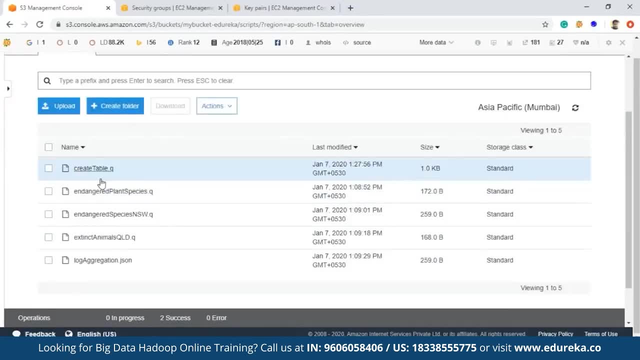 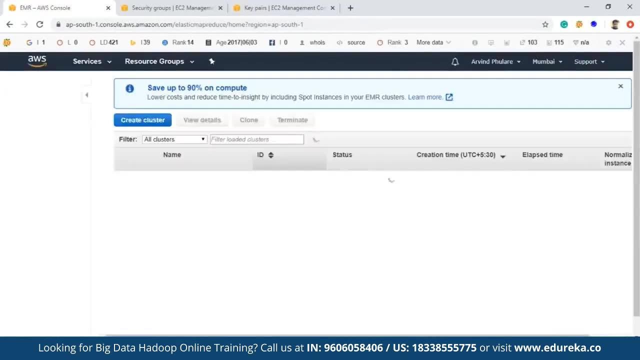 s3 bucket. So, as you can see here now we have four queries here and one Jason file. So let's just quickly go back to our cluster here And we just need to add one step here. like for executing for queries, We'll be needing four steps. 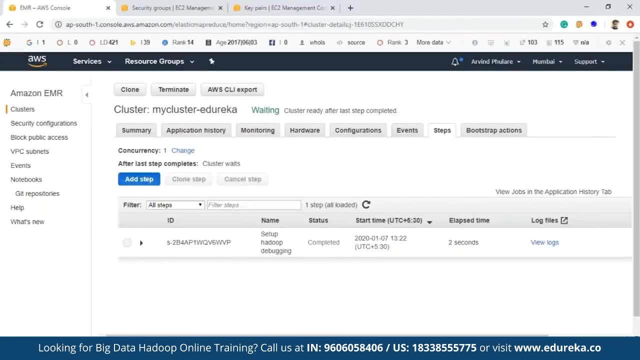 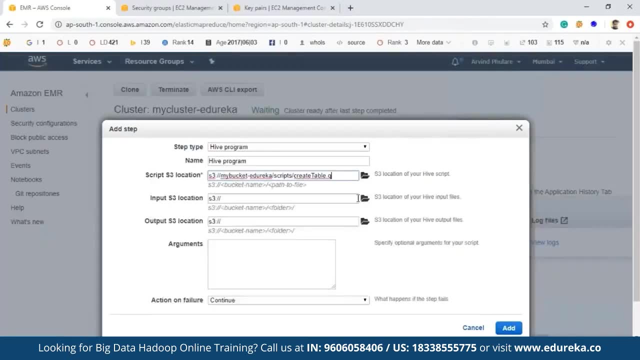 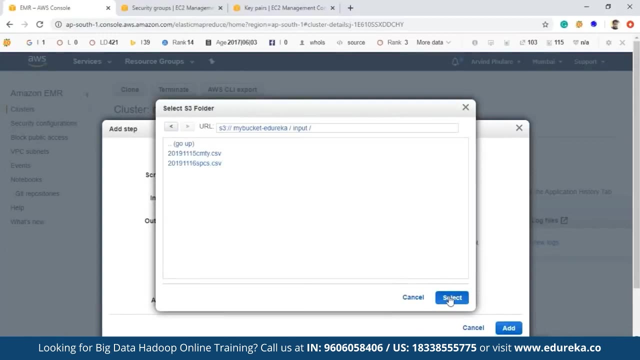 So if you click on this step section, click on add step, Select hive program, select the script location, create table. Okay, So the input for this is the CSV files which are stored on the input folder of our bucket. Once you do that, select the input folder- select the output folder as well. 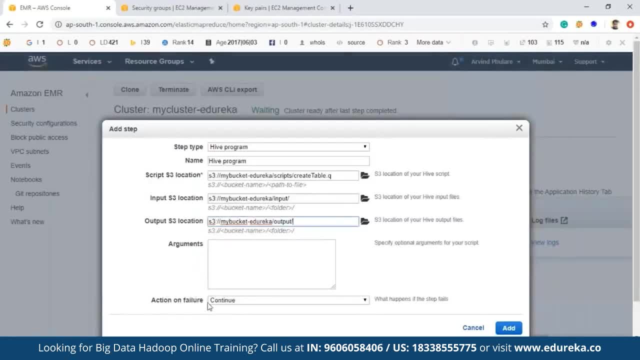 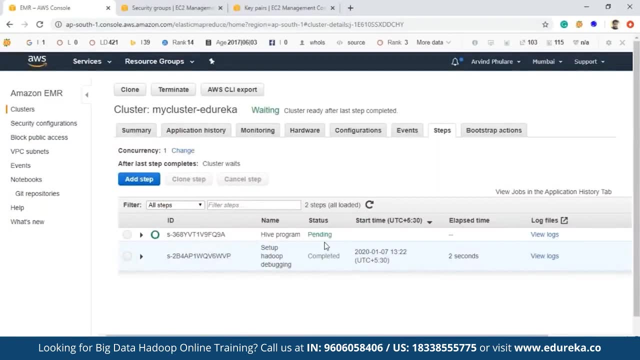 Okay, so this is the default action on failure: continue. Okay, click on add here. So running this step might take a few seconds. As you can see here, the status is pending and once this status turns from pending to completed, we will add remaining steps in a similar way. 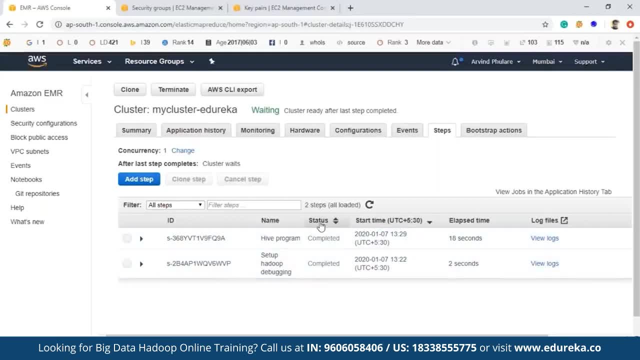 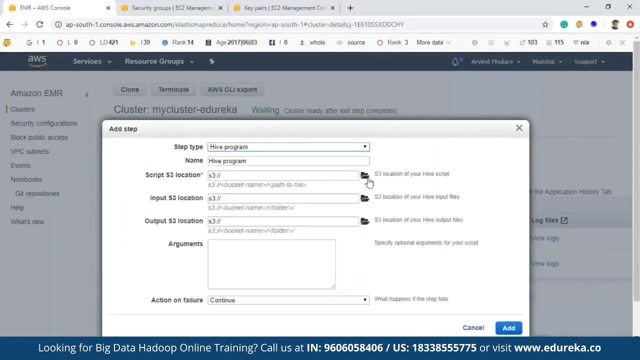 Okay. so, as you can see here, the status has changed from pending to completed. So similarly, for remaining queries you have to add steps in the similar way. So the type program, select the script location. We will add the input, The input. 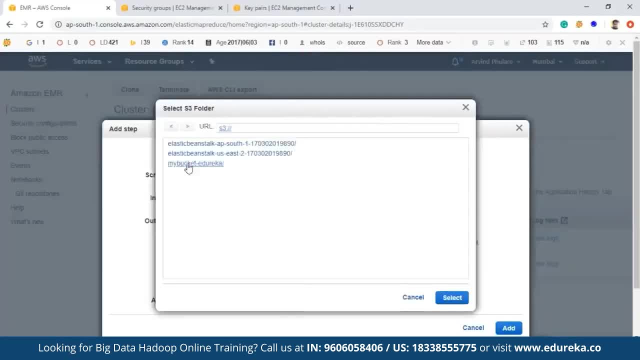 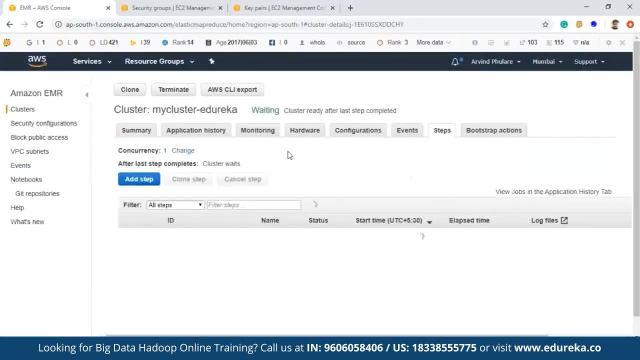 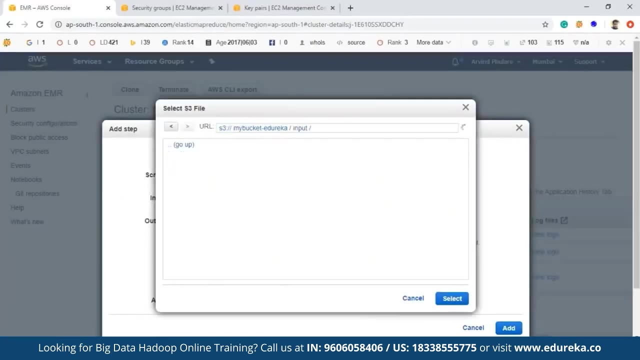 And the output. Click on add and let's just quickly add two more steps here And we will also have a look at the output after these queries are successfully Executed. I'll show you how do you view the output of this queries. 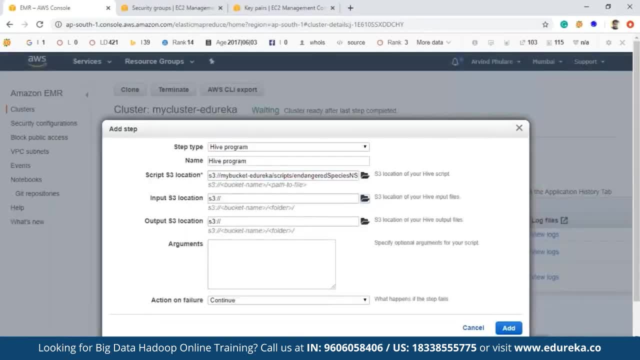 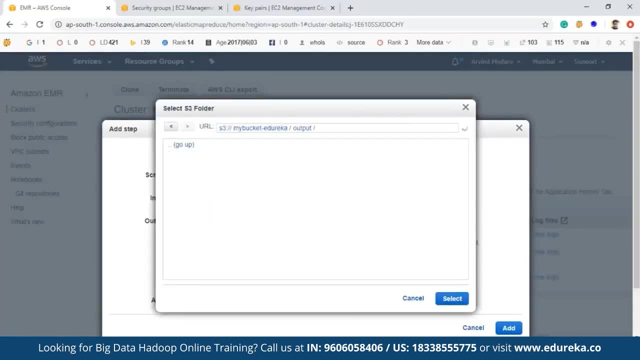 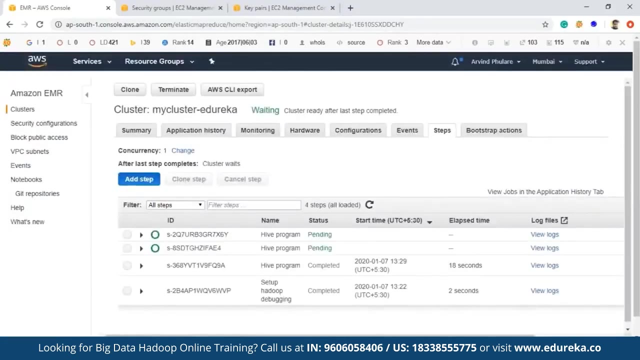 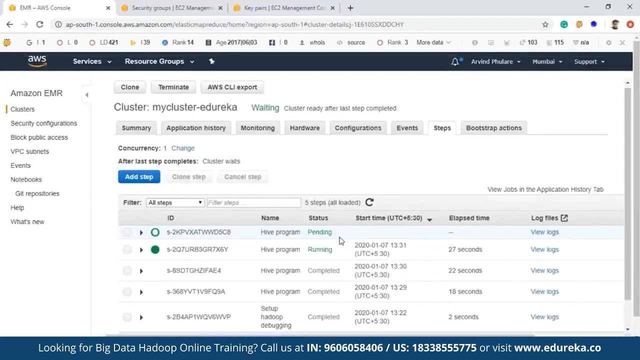 Okay, So now let us just quickly select the input And the output, Click on add and we'll just add. one last step for the fourth query. Okay, so, as you can see here, two queries have been successfully completed and the status of the remaining two queries- one- is pending. 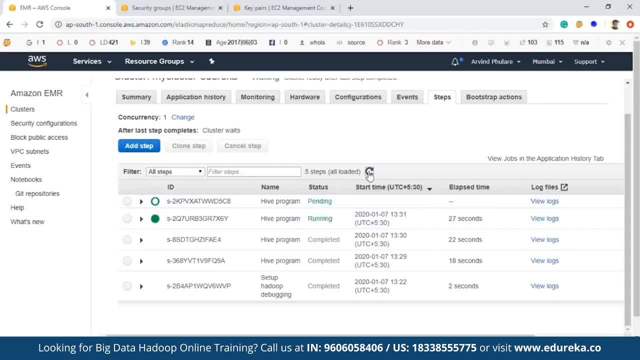 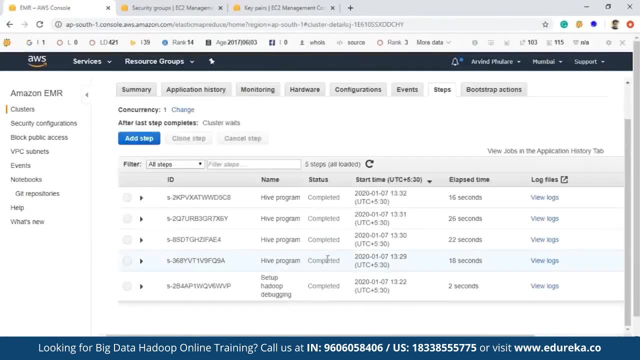 and one is running. Okay, so, if you refresh this. Okay so, as you can see here, we had four queries and all the four queries have been successfully executed. Okay, so this is how you execute your high queries on the top of your data using the EMR cluster. 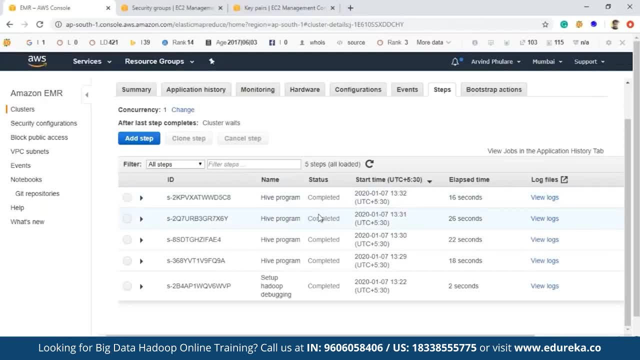 So, guys, with this we have come to the end of this session on big data in AWS and I hope you have enjoyed this session and you have understood whatever we have done here. If you have any queries related to this session, you can post them in the chat box below. 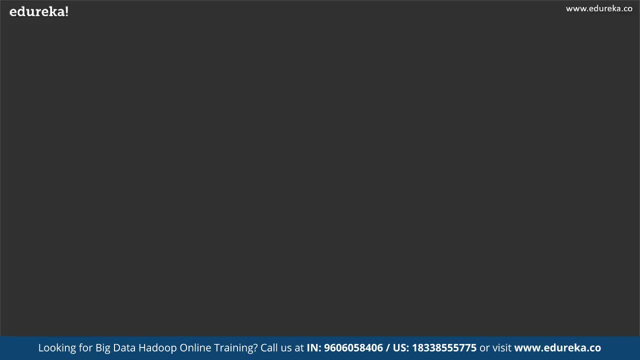 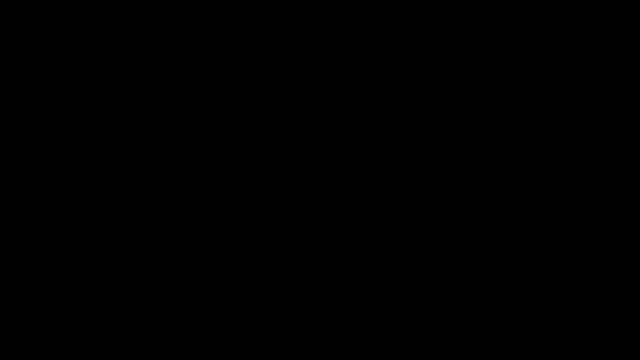 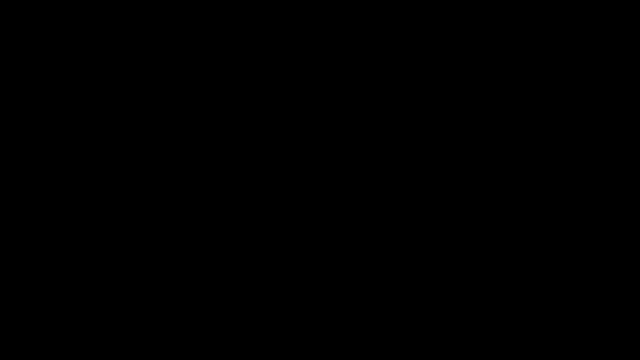